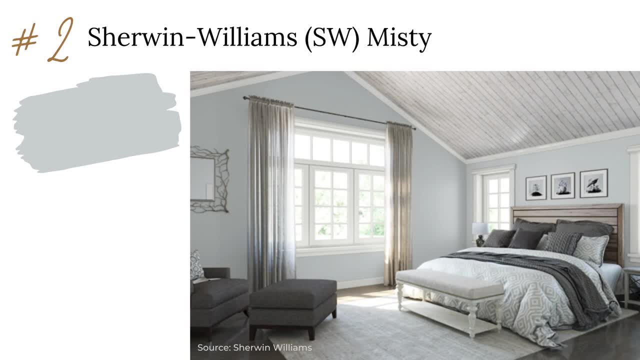 blue than Quiet Moments does. The great thing about Misty is that even though it's a light blue, it has enough gray and even just the slightest hint of green in it to look very nice and sophisticated. In certain lighting it's going to look very gray and neutralized, while in other 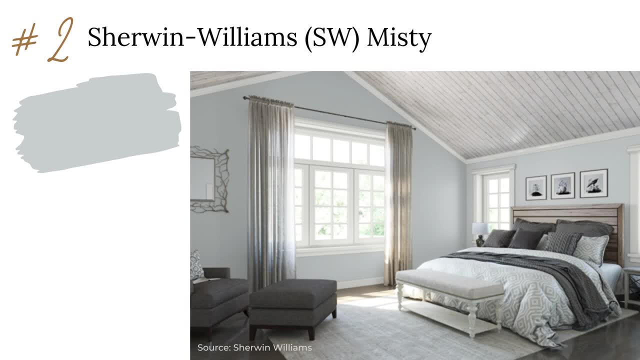 lighting conditions it could look a little more blue. You should pair Misty with whites and grays or even darker blues, and include some warmer elements like wood to help soften the look. Sherwin-Williams Krypton is number two. It's a little bit lighter, but it's a little bit more. 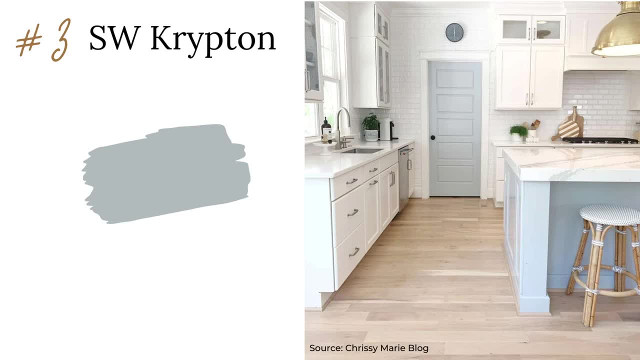 colorful Number three. Now Krypton is on a paint strip with some other really popular blue-grays. The reason these colors are so popular is because they're just all perfectly balanced blue-grays and they tend to look gorgeous wherever they're used. So check out this beautiful kitchen with. 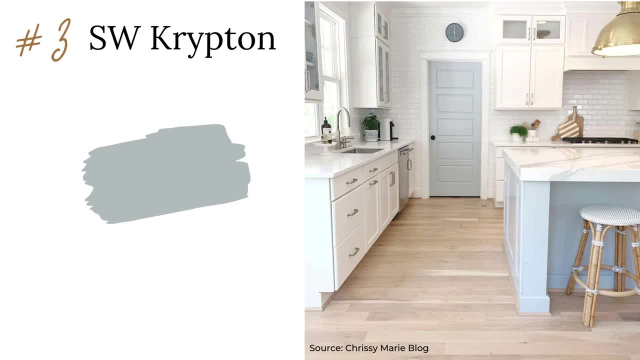 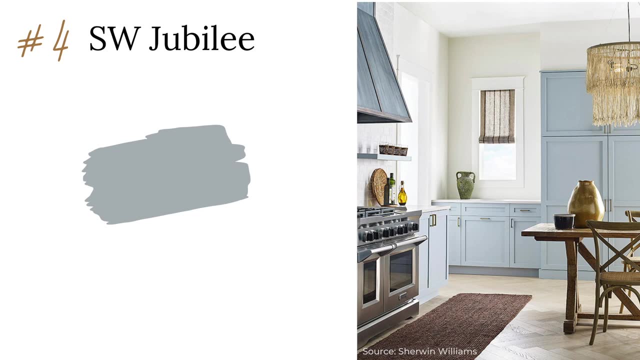 the island and pantry door painted with Sherwin-Williams Krypton. It's a really gorgeous coastal vibe. Number four is Sherwin-Williams Jubilee. Now you know how I just said that Sherwin-Williams Krypton was on the same paint strip with other fabulous blue-grays. 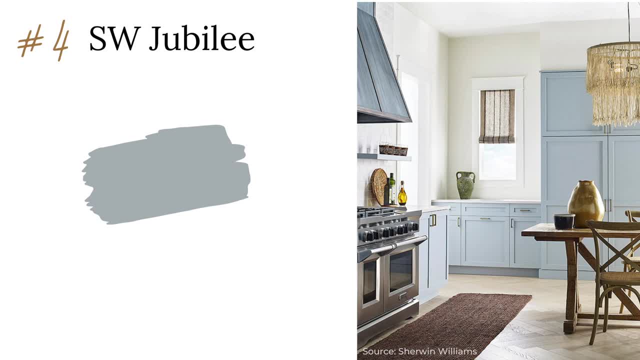 Well, Jubilee happens to be one of them. Jubilee is just about one shade darker than Krypton, but so fantastic that it deserved its own spot on the list. This medium blue-gray looks really beautiful in any room and a great place to start when you're sampling blue-gray paint colors. 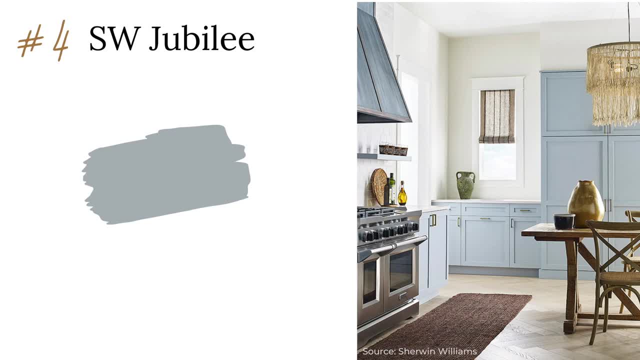 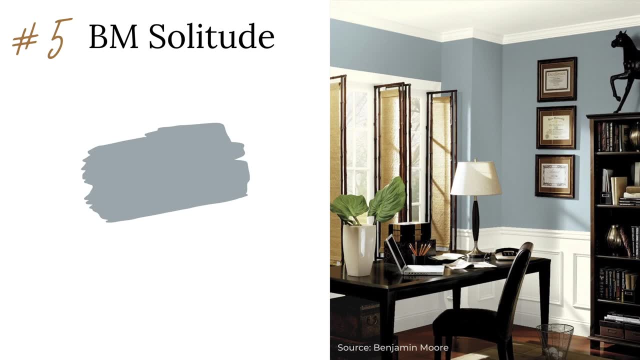 Just look at how beautiful Jubilee looks on the cabinets in the kitchen picture here. Number five is Benjamin Moore's Solitude. Now, as we venture into more of the medium blue-grays, Benjamin Moore's Solitude is definitely one of the most popular blue-grays in the world. 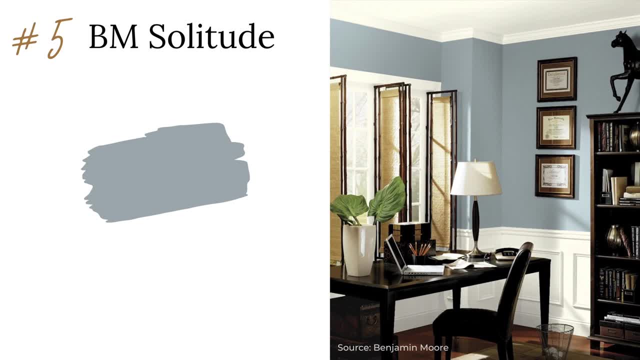 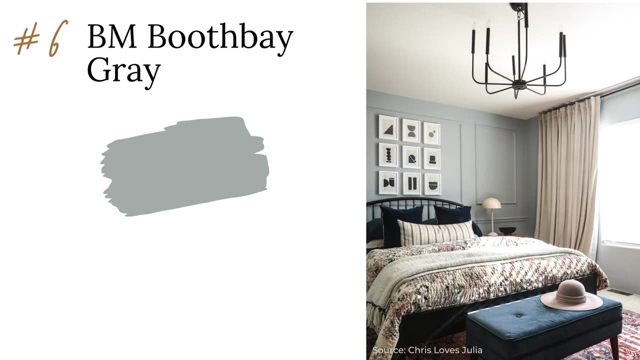 Number six is Benjamin Moore's Boothbay Gray. Boothbay Gray is one of my all-time favorite blue-grays because it just looks amazing wherever it's used. It's a bit of a chameleon in that it can look much more gray or much more blue-green gray, But it's a beautiful, classic popular paint color from Benjamin Moore and worth a sample for sure. 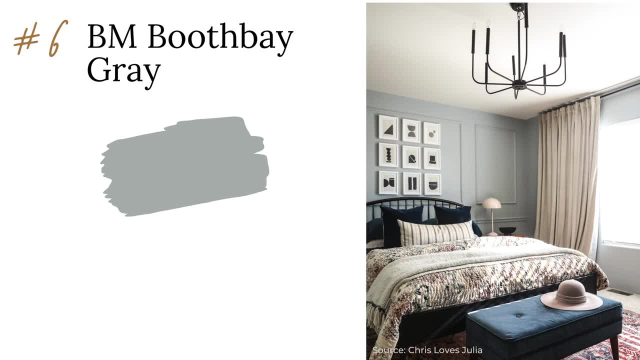 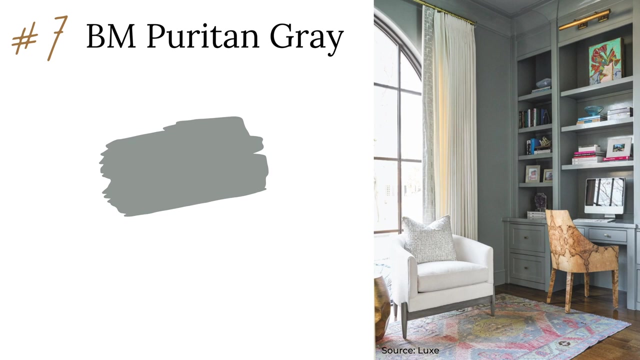 Number seven is Benjamin Moore's Puritan Gray. This is another historical color from Benjamin Moore and it's a little darker than Boothbay Gray and has a bit more green to it. It's really beautiful on cabinetry indoors and can be a very soothing color in an office or bedroom. 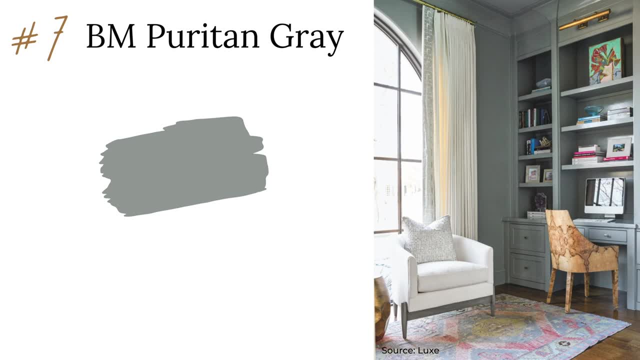 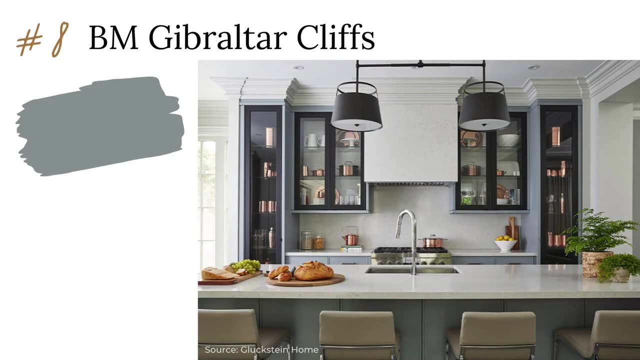 If your blue-gray is shifting to blue or purple in your space, give Puritan Gray a try. Coming in at number eight is Benjamin Moore's Gibraltar Cliffs. This is a medium blue-gray and it's really closer to a gray but has some serious blue undertones. that will really show. 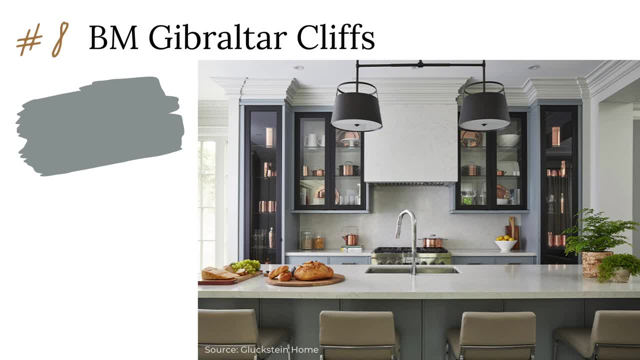 themselves once you paint. You want to pair Gibraltar Cliffs with soft whites to keep things light and airy and warm- elements like wood. You want to pair Gibraltar Cliffs with soft whites to keep things light and airy and warm- elements like wood. You want to pair Gibraltar Cliffs with soft whites to keep things light and airy and warm- elements like wood. 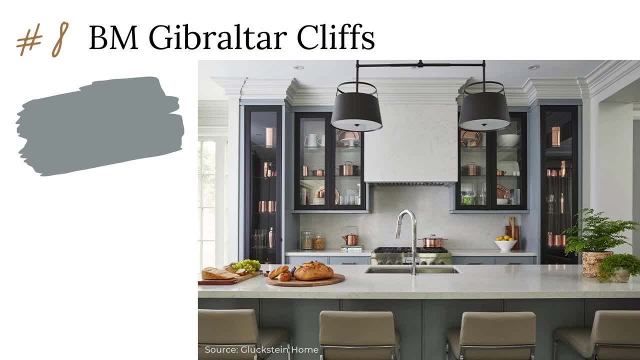 You want to add some more different accents like silver, brass or copper to help balance out the coolness of this color. You want to add some more different accents like silver, brass or copper to help balance out the coolness of this color. 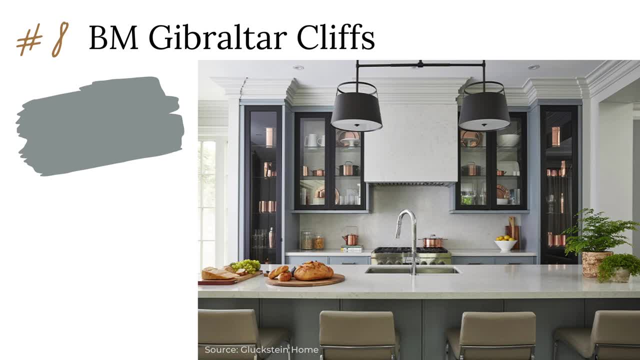 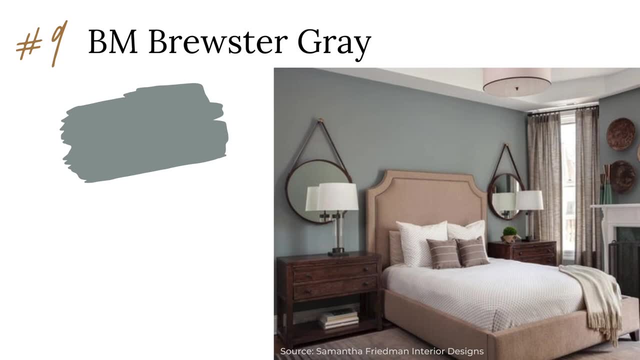 This kitchen's a beautiful example of all of those elements working really well together. Number nine is Benjamin Moore's Brewster Gray. Brewster gray is another timeless hue from Benjamin Moore's historical collection. It's a medium dark blue-gray that is quite elegant and 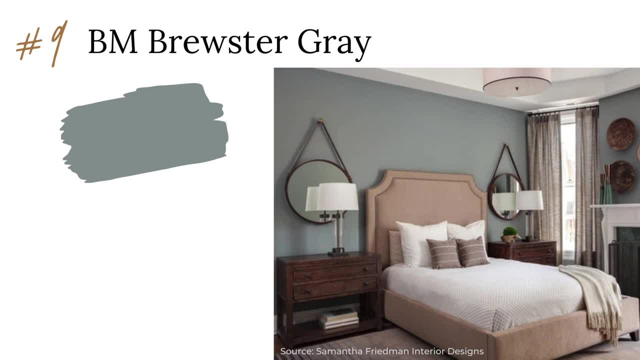 pairs beautifully with rich wood furniture pieces. due to its subtle green undertones that it has Now, Brewster Gray is a great choice for bedrooms. It's not too light, it's not too dark And it will be a great choice for your bedroom For sure. if you're looking for a big mirror, you'll love this color. 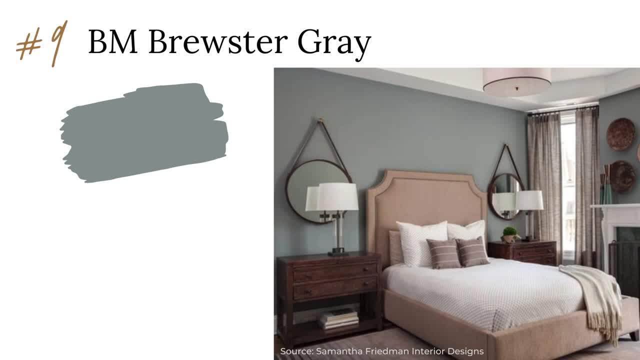 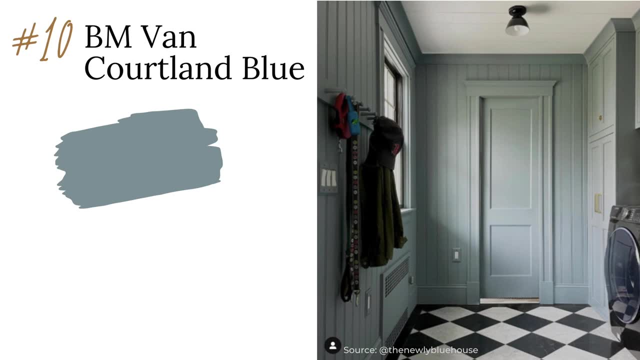 will look fantastic if you have darker stained wood floors or darker wood furniture in your room. Benjamin Moore's Van Cortlandt Blue comes in at number 10 and it's been a really popular blue gray paint color for years. On the paint chip it looks like the perfect blend of blue and gray, but 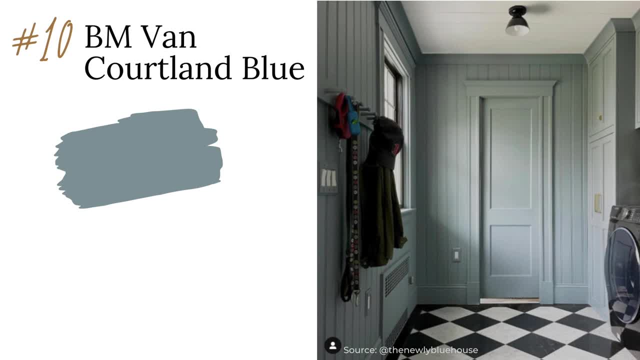 just know that it can tend to look a little more saturated and blue than expected when you paint it on the walls. I recommend googling images of Van Cortlandt Blue to see the many variations of this color, and always sample the color on your walls before committing. Check out this fabulous. 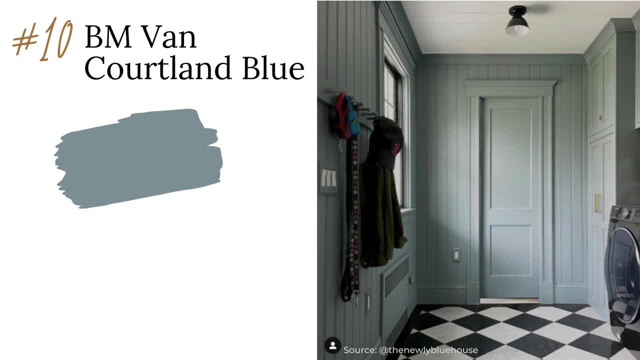 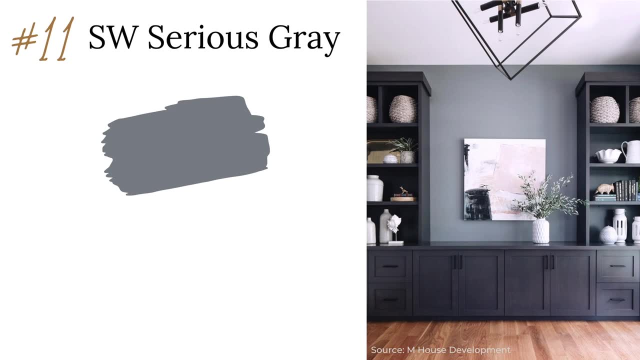 laundry room showcasing Van Cortlandt Blue on the walls, doors, cabinetry and trim. Number 11 is Sherwin-Williams Sirius Gray. This is a medium dark gray with blue undertones. Depending on your lighting, Sirius Gray can look very gray because its blue undertones are a little bit more subtle. 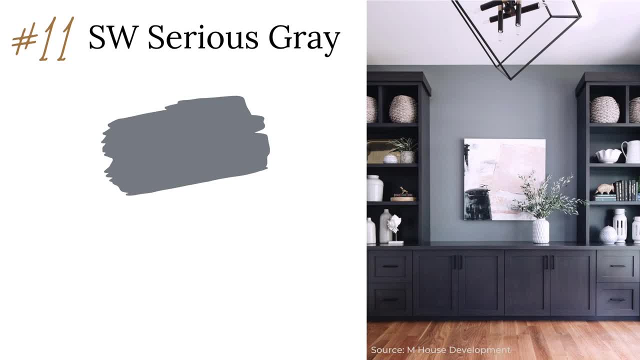 than some others on this list. I love using Sirius Gray for cabinetry and exteriors and it works best in well-lit spaces, But it can also be a good option for creating that dark, moody feel in a den or office. You can see how. 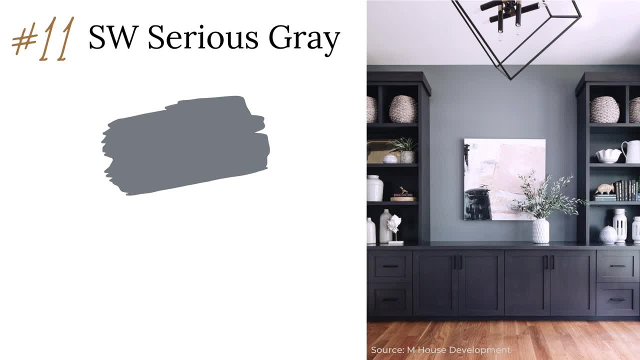 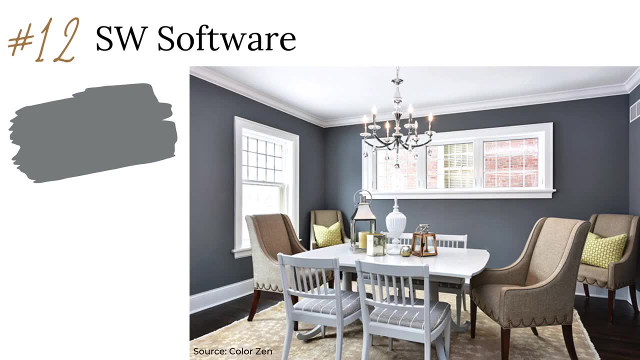 pretty. Sirius Gray looks here as an accent wall and backdrop with the built-in bookcases. Number 12 is Sherwin-Williams Software. Like Sirius Gray, Software is another medium to dark, cool gray with blue undertones. Because it's fairly dark and very gray, I recommend pairing software with lighter. 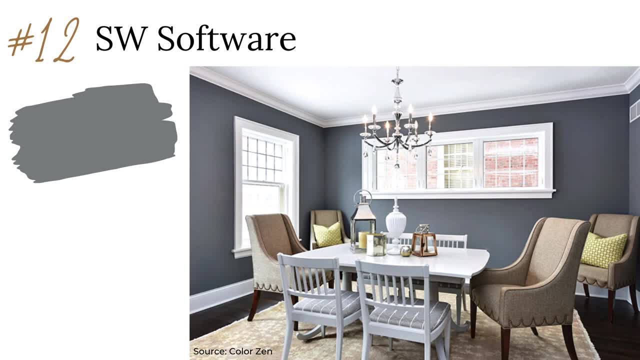 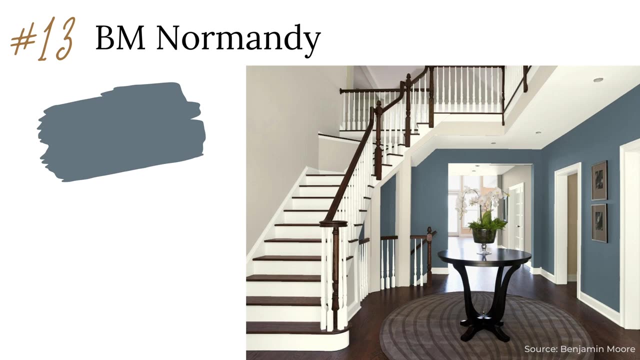 wood tones and crisp whites, And it also works great with pinks and blues. Number 13 is Benjamin Moore's Normandy. This is a classic medium to dark blue gray that leans slightly more toward the blue side. It's a great color for traditional homes and it's a solid choice for an office. I've seen it used on kitchen cabinets and it's quite blue, But it could be a fun way to make a statement in your kitchen. In this entryway, Normandy makes a great statement and provides visual contrast to your home. 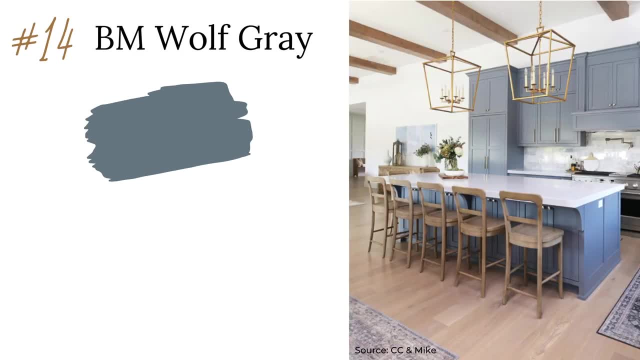 with the other wall colors. Wolf Gray by Benjamin Moore is number 14 on my list, and this is another medium to dark gray with cool blue undertones. It's become one of my favorites for both interiors and exteriors, because it strikes a beautiful balance between its gray and blue tones and it 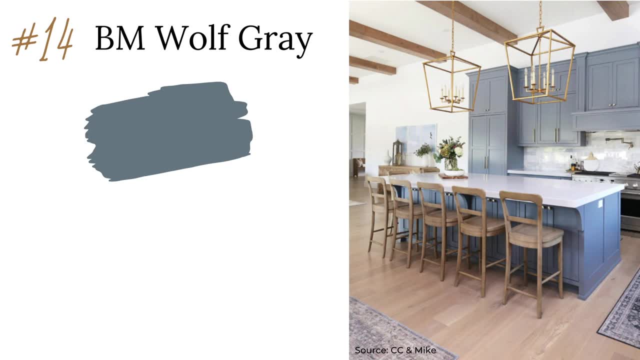 works really well paired with a wide range of colors. Wolf Gray looks equally gorgeous on kitchen and bath cabinets as it does on bedroom walls. Here's a lovely kitchen showing Benjamin Moore's Wolf Gray on the cabinets. Sherwin-Williams Smoky Blue is a darker blue gray with some teal. 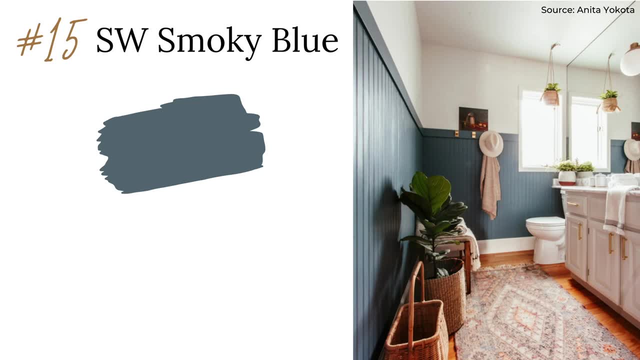 undertones and it comes in at number 15 on my list. It can be a nice dramatic shade for an office or dining room, but it's more saturated than other blue grays that I would normally recommend for cabinetry. You can take a look at this adorable boho bathroom with Smoky Blue on the wainscotting.